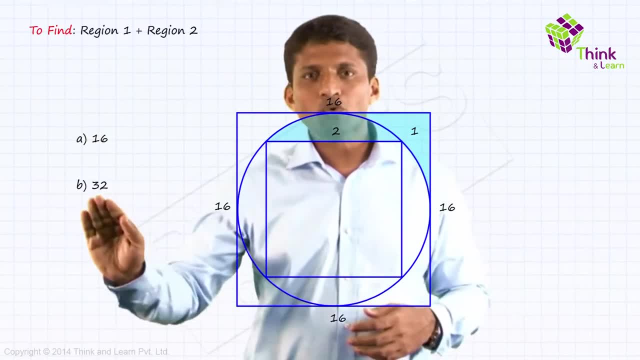 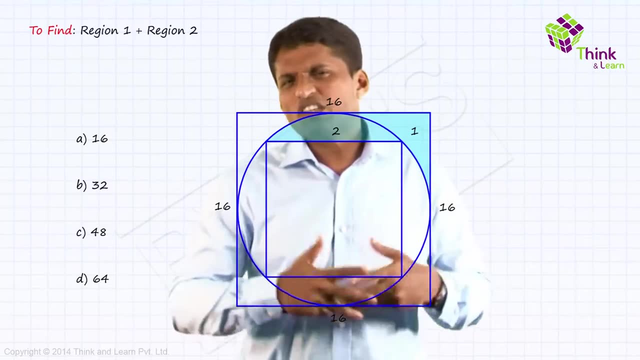 I'll also give you answer options, which are 16,, 32,, 48,, 64. And if I give you time, I'm very sure, given time, all of you will solve this question And there is a very good chance that 99% of you are solving it this way. 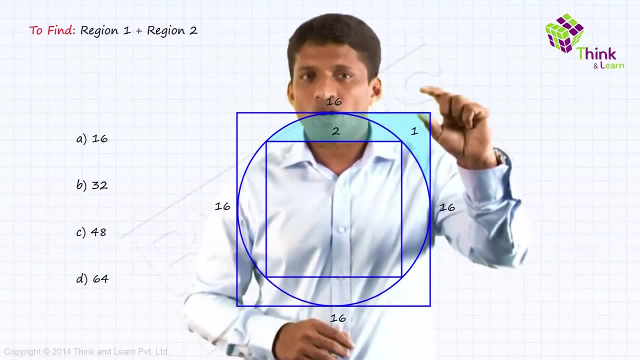 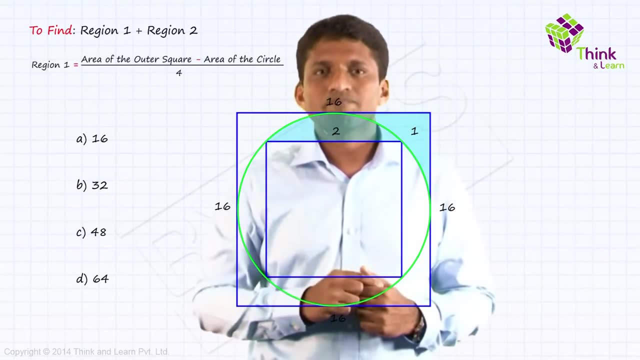 And how will you solve Region 1.. How will you find region 1?? Region 1 is area of the square minus area of the circle, And you'll divide it by 4.. Now, why are you dividing it by 4?? 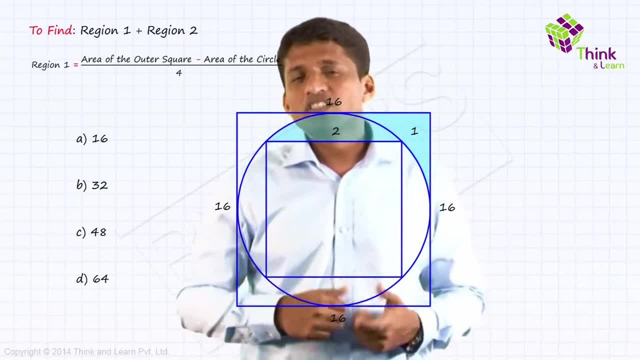 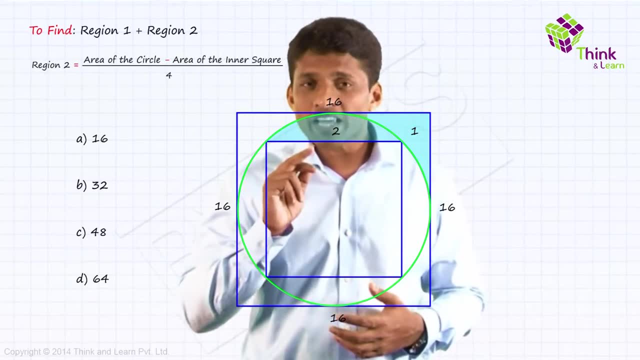 As you can see, there are 4.. That's why we are saying equal regions. Same way, how will you find region 2?? Region 2 is area of the circle minus area of the inner square, And there again you will divide by 4.. 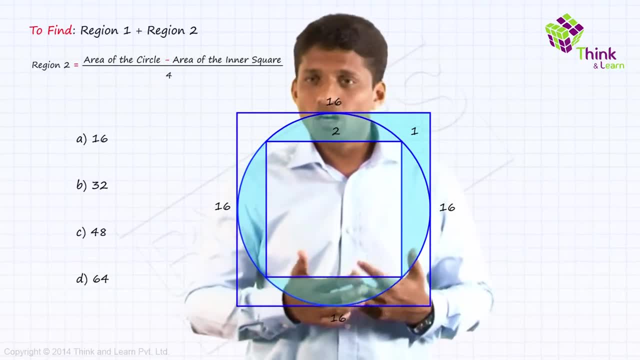 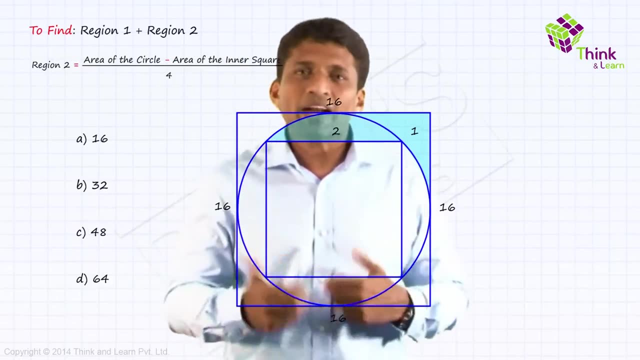 Because, as you can see, there are 4 regions like 2.. Now, when you are doing this, pi is involved in calculation. because circle is involved, Options are without pi. That's why you'll end up taking one and a half, two, two and a half, three minutes. 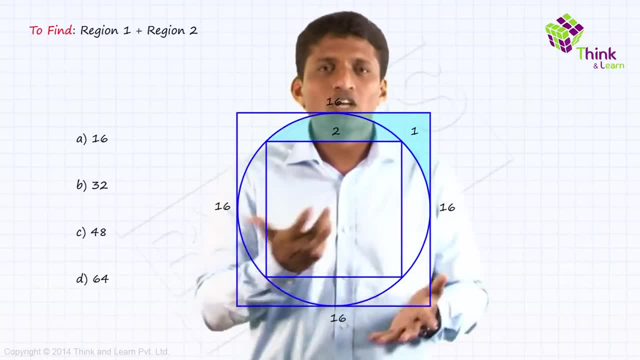 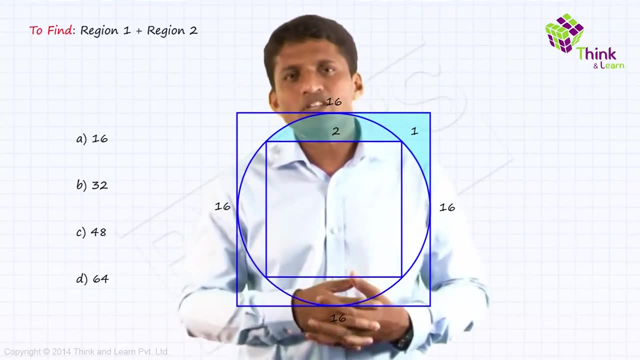 depending on your calculation speed- Whether you're fast, super fast, average. That will decide how much time you will take to convert this into the answer options. So I'm sure you will get the answer. This is the original question. 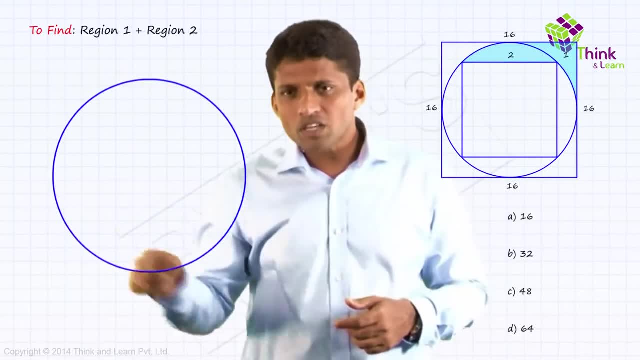 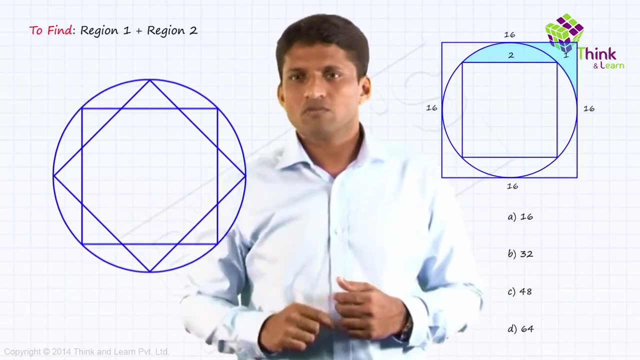 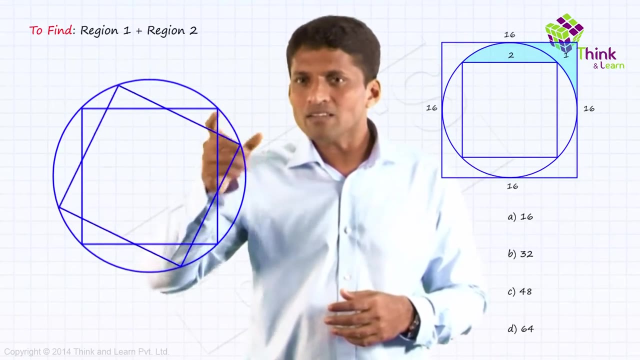 Now, if I ask you a question back, take a circle, whether I take a square like this or whether I take a square like this, can I take any square? can I take any square here? I'm just changing the orientation. I'm simply rotating the first one square to get the second one. 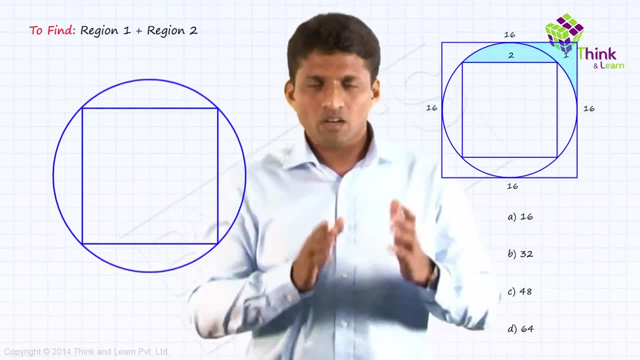 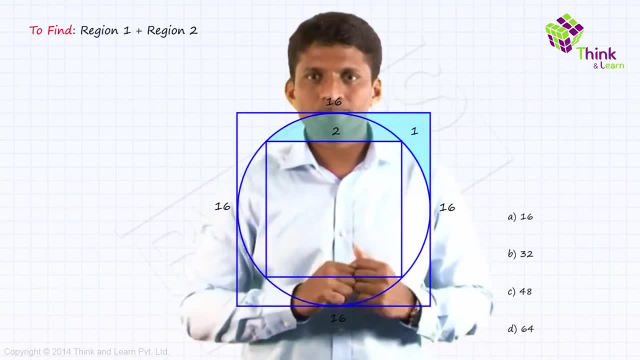 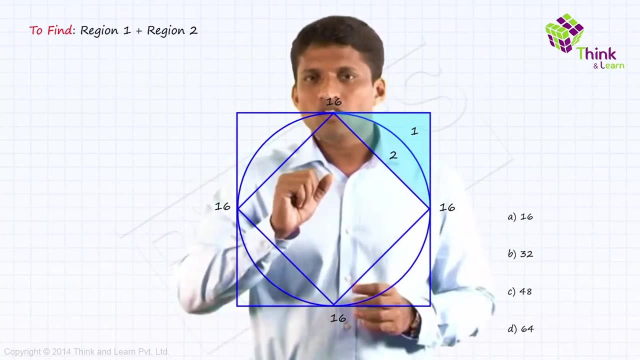 Now, if I use the same logic or same common sense to solve this question, what we'll get is: so let's look at the original diagram. This is the diagram. The regions are shaded one and two. Now the inner square. if I just rotate like this, what is happening? 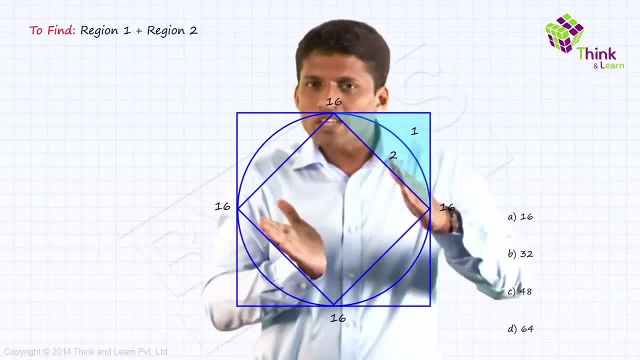 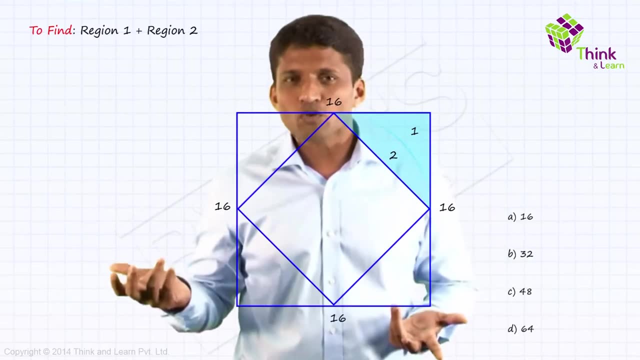 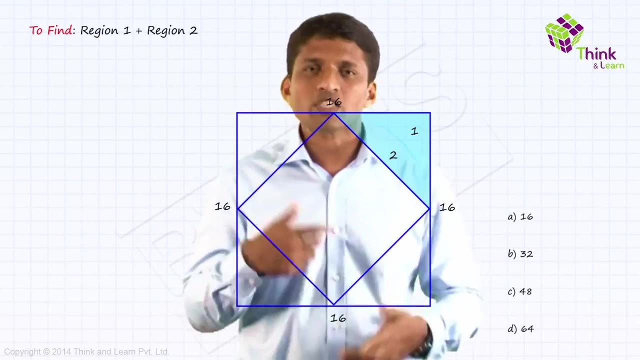 You get region one here, you get region two here. Now they are together. So now it's an advantage because circle is out, So pi is out of calculation. Now it's not a question. It will become well below our level At its lowest level. if you want to solve how we are supposed to solve. 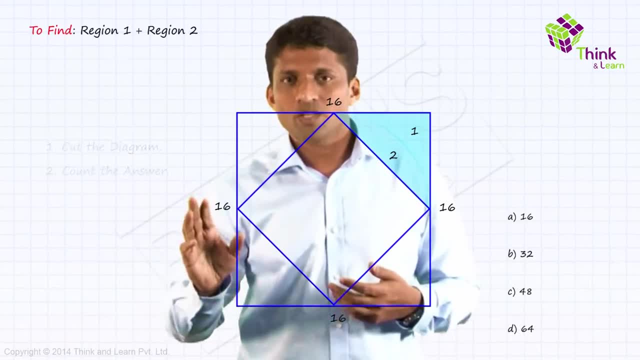 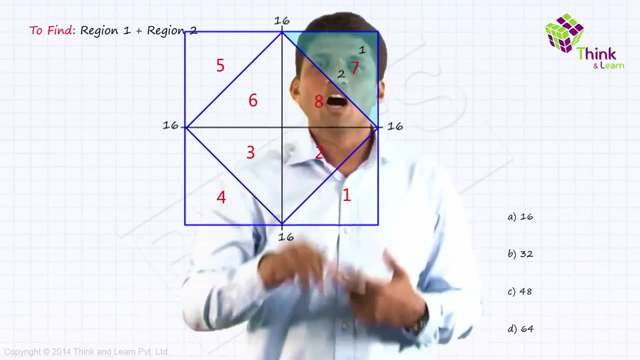 I'll write in two words: cut the diagram and count the answer. Cut the diagram like this and count the answer: 1,, 2,, 3,, 4,, 5,, 6,, 7, 8,, out of which only.